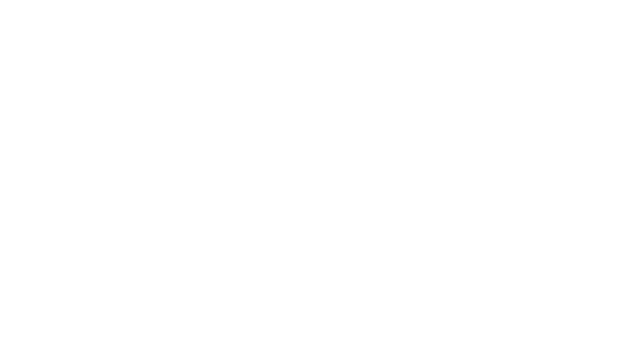 So in this lesson we are going to learn how to find the general solution to a second order linear, non-homogeneous differential equation with constant coefficients. So previously we got to understand that a second order linear differential equation is given of the form p of x times y prime prime plus k of x times y prime plus r of 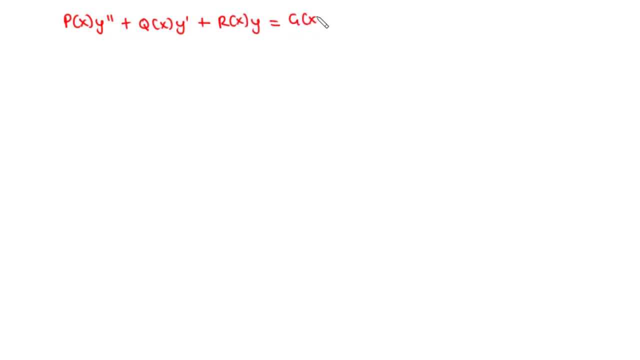 x times y equals g of x. Now if p of x, k of x and then r of x are said to be constant coefficients, then basically we are going to represent each of them with a constant. So we say that let p of x be equal to a, k of x be equal to b and then r of x be equal. 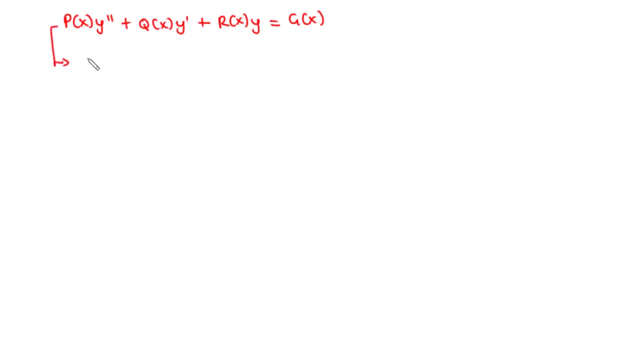 to c, so that we have the differential equation expressed as a: y prime, prime plus b of x, dy prime plus cy equals g of x, where g is said to be a function of x or, better said, a continuous function of x. Now, if g of x is equal to zero, then we have a homogeneous 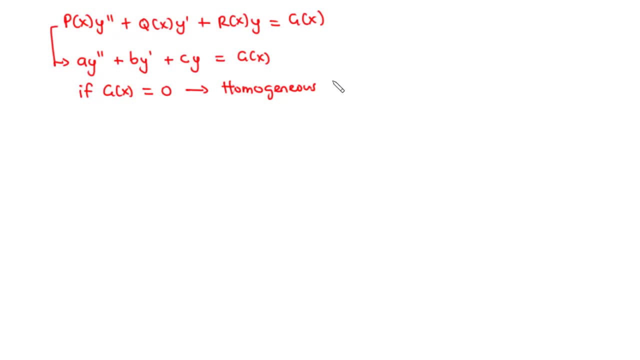 differential equation, a homogeneous differential equation. And if g of x is not equal to zero, then we say that we have a non homogeneous differential equation. and that is where our interests lie. we want to find the general solution to a second order linear, non homogeneous differential equation with constant. 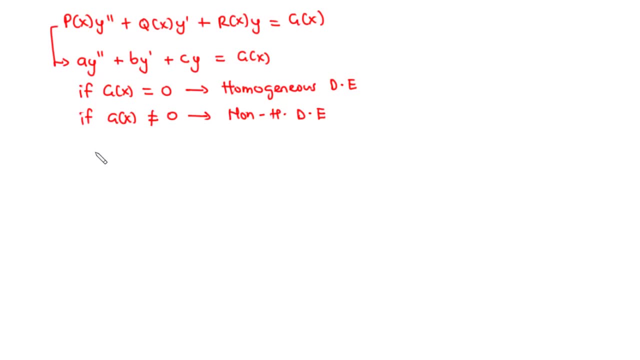 coefficients. now, the general solution to a second order linear, non homogeneous differential equation is given by Y equals Y C plus Y P, where Y C is said to be the complementary function- complementary function- and then Y P is said to be the particular integral, particular integral. so, in effect, what this primarily means is that, given a second order linear, 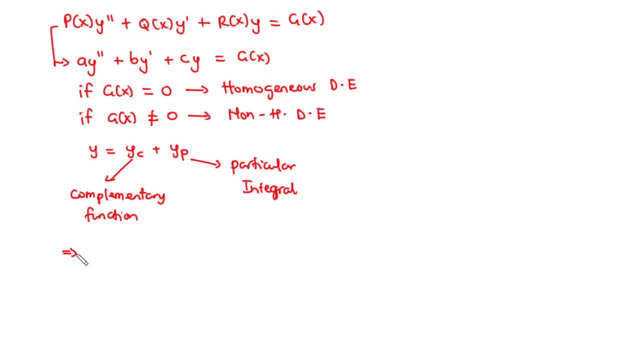 non homogeneous differential equation with constant coefficients of the form a- Y prime prime plus B. Y prime plus C. Y equals G of X, where G of X is not equal to zero. the first thing we are going to do is to find the general solution to a second order linear, non homogeneous differential equation. 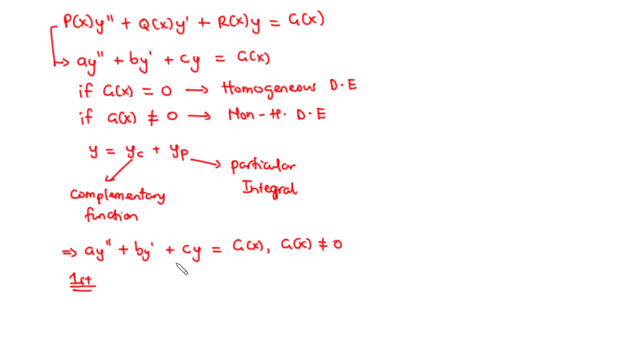 the first thing we are going to do is to treat the given differential equation as a homogeneous differential equation, that's by making G of X equal to zero. so you are going to have a Y prime prime plus B, Y prime plus C. Y equals zero. so it 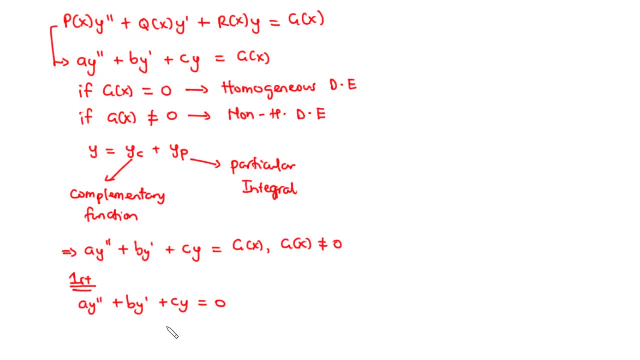 becomes a homogeneous differential equation. and you try to solve the general solution of this homogeneous differential equation, and that is given by Y C, which we call the complementary equation, and that is given by Y C, which we call the complementary function. and then the second step is to solve for the 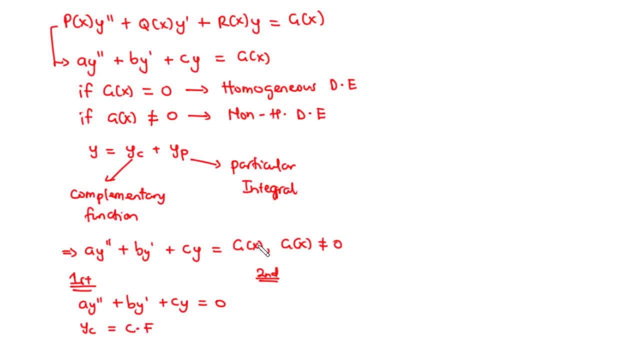 particular integral. so for the particular integral, we are going to focus on the non-homogeneous them, which is G of X, the function on the right hand side. so you focus on G of X and learn, you derive the particular integral. now the particular integral is said to be Y, p, and then the particular integral can be. 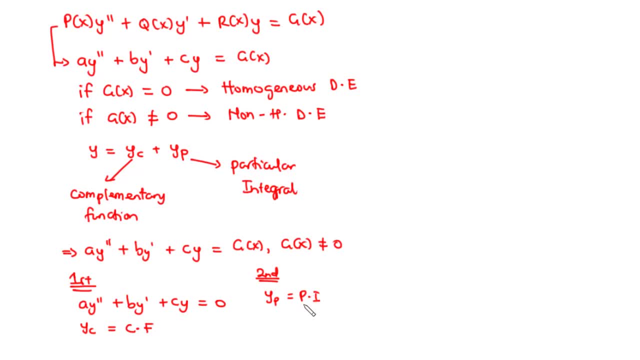 be determined using the method of undetermined coefficients. So at the end you have the general solution to the given differential equation, to be equal to or to be given as: y equals yc plus yp. Also notice that the nature of the particular integral also depends. 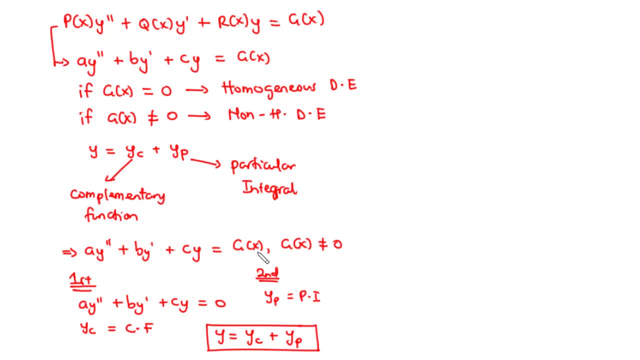 on the function g of x. So if you have a polynomial, a constant, an exponential function, all are going to take different formats. So in this lesson we are going to focus on, when g of x is equal to a constant, how to find a particular integral and hence how to find: 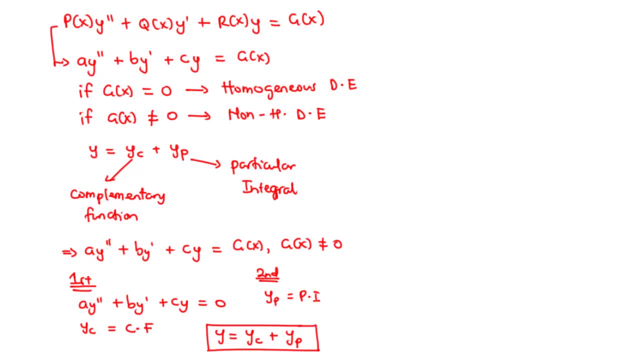 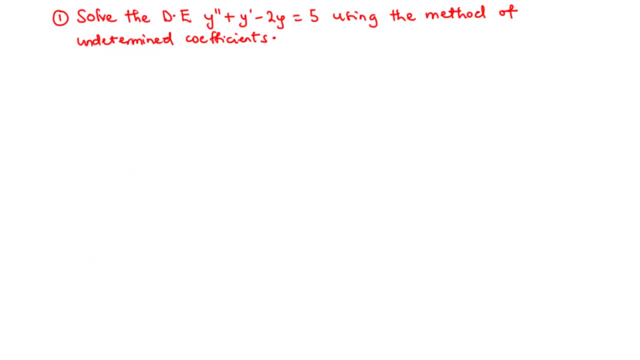 the general solution to the given differential equation. Now let's take our very first example. So in our first example we are asked to solve the differential equation y prime prime plus, y prime minus two- y equals five- using the method of undetermined coefficients. 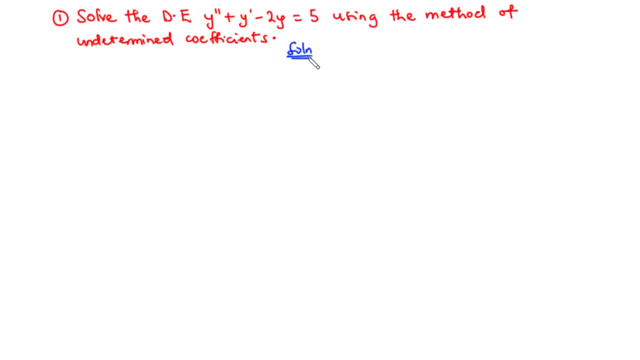 so let's try to solve this problem together. so we have the differential equation: y prime prime plus y prime minus 2y equals 5. now this is a second order linear, non-homogeneous differential equation with constant coefficients. now, the first thing we are going to do, the first thing we are, 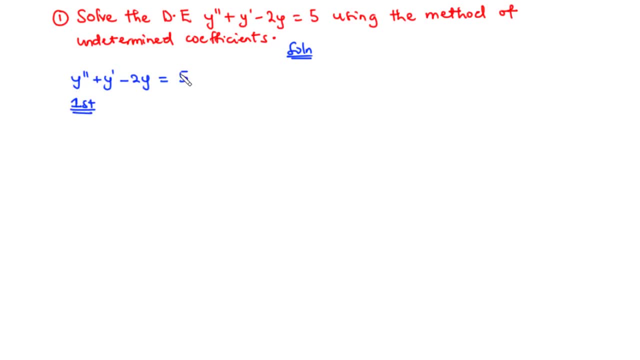 going to do is to treat this differential equation as a homogeneous differential equation. so by so doing we are going to make the right hand side be equal to zero. so thus we have y prime prime plus y prime minus 2y equals 0. so this time we have a homogeneous differential. 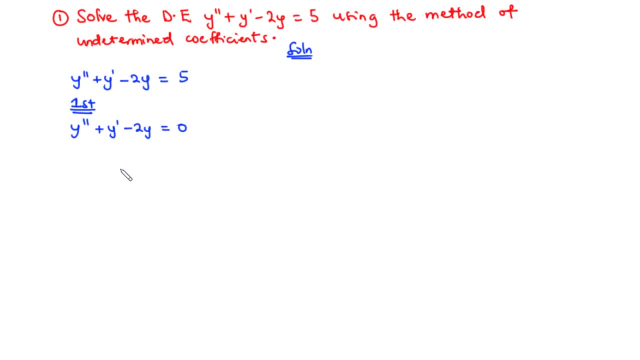 equation and let's try to obtain the auxiliary equation or, better still, the characteristic equation. so from this you remember that you will be getting the 2y equals 0. we are going to represent y, prime, prime with M, square y, prime with M, and then y. 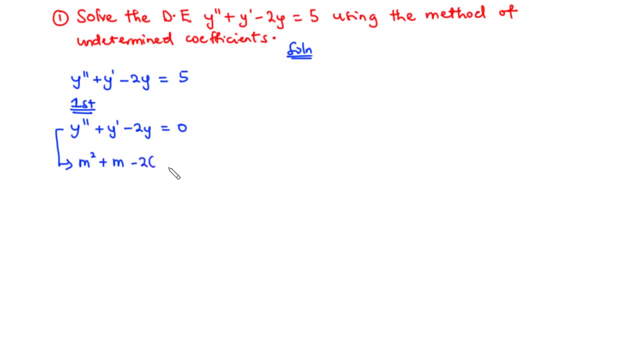 with 1. so negative 2 times 1 is still negative 2 and that's equal to 0. at this point you can find the roots of the auxiliary equation. so we multiply the coefficient of M square and then the coefficient of the constant we have. 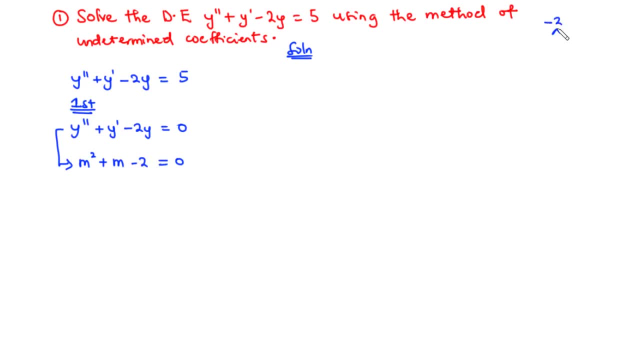 negative 2. and then we want to find two numbers that when you multiply you are going to obtain negative 2, but when you add them you are going to obtain 1. so we have negative 1 times 2. so negative 1 times 2 is negative 2. negative 1 plus 2. 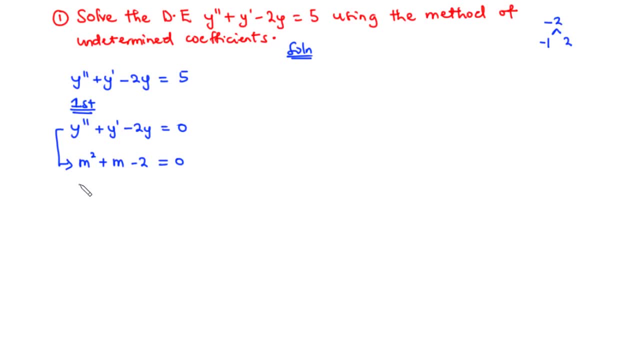 is 1. so we have the factors to be: M minus 1, and then M plus 2 equals 0. so M minus 1 equals 0. we have M equals 1, and then M plus 2 equals 0. we have M equals negative 2. so let's call this m1. 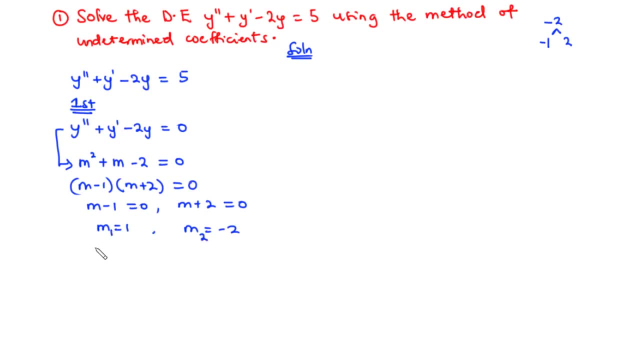 and let's call this m2. so here we have two real end on equal roots or, better still, two real-end the extinct roots. so the general solution to this homogeneous differential equation is given by Y. C equals C 1, e to the power, M 1 X plus M1 x- T 1.. Since C1 is equal to a호�, Are we going to have negative 2? so here we are putting negative 2 or or equal to m2, and so it's so simple. so we are putting M 1 x plus m2, equal to R. andolwall hall is equal to negative 2. so lettuce call this M1, and let's call this m1, and let's go this him too. so let's McGarrett. so here we have to to maar e to the power M1, x plus he evens x to the power mone, x plus m17. and then we have two real end to grey and v. then we have 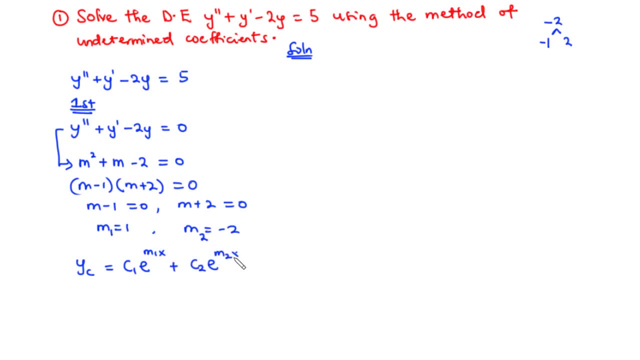 c2 e to the power m2 x, so that we have c1 e to the power m1 is 1, so 1 times x is x plus c2 e to the power m2 is negative 2, so negative 2 x, so that is the complementary function. 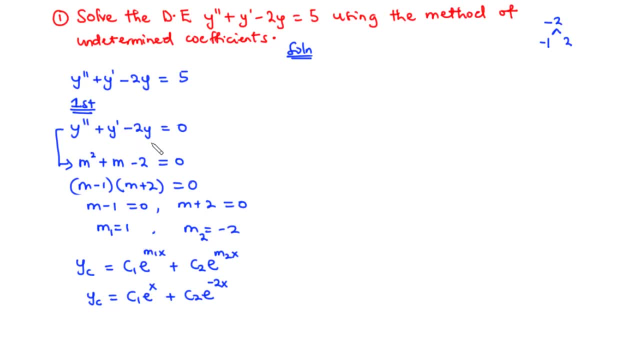 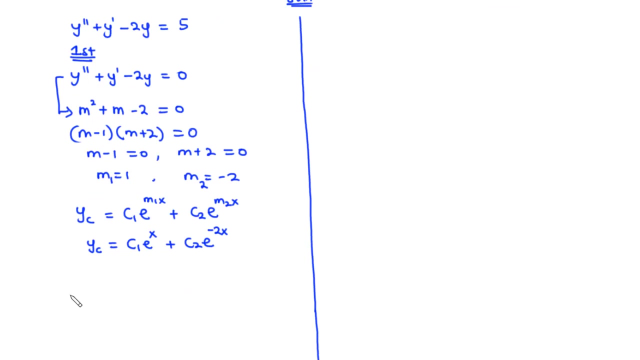 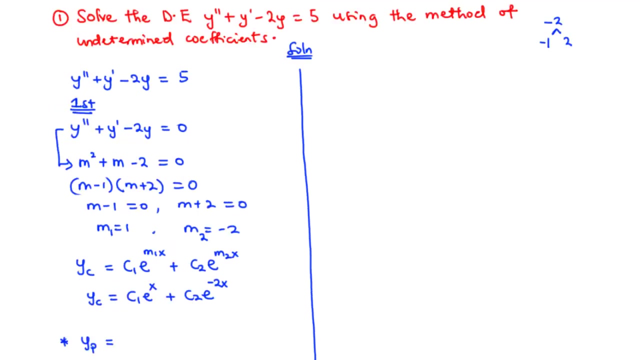 the general solution to the homogeneous differential equation. so at this point let's try to find the particular integral. so for the particular integral, we are going to say that the particular integral is equal to. now, before we can know what the particular integral is equal to, we need to focus on the function g of x. so this is g of x. 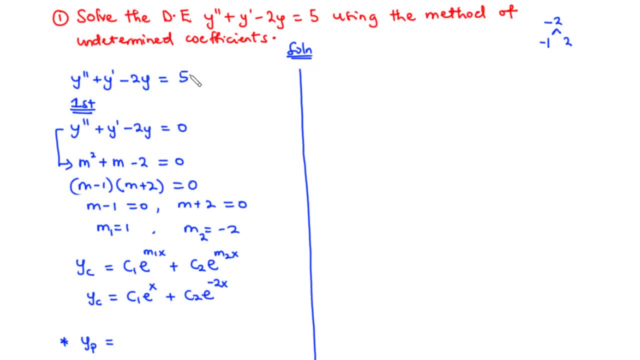 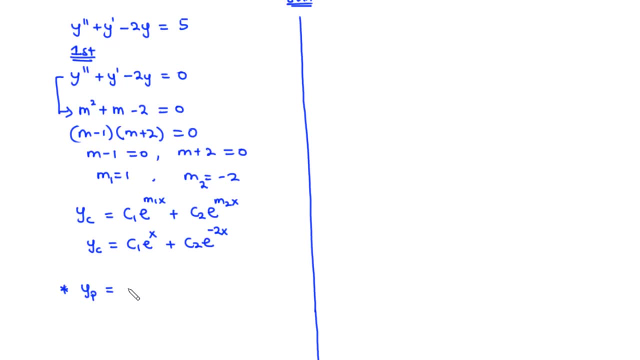 so we are going to say that the integral is equal to. so g of x here is a constant. now, so long as g of x is a constant, then we say that yp is equal to a. so if we have a constant, then we are going to deploy. 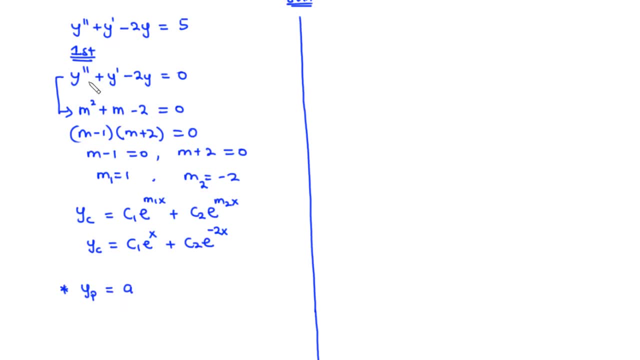 yp equals a. now looking at the differential equation, we have y prime prime and then y prime. so let's try to find y prime prime and then y prime from this equation. so we have yp prime. when you differentiate a constant, you have zero, and then we have yp prime, prime. 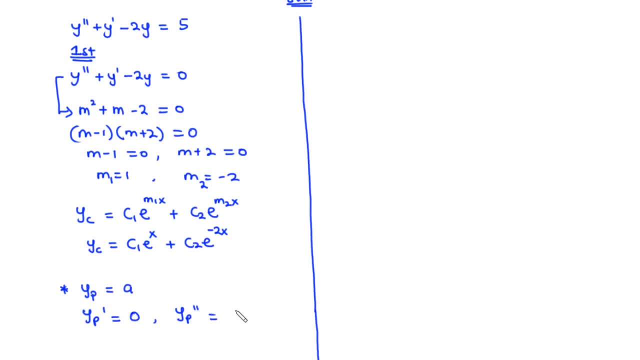 again, when you differentiate, a constant, zero is a constant, it becomes zero. so at this point we are going to plug in the values yp, yp prime, yp prime prime, in place of y prime prime, y prime and then y. so for this differential equation we have y prime prime, which is zero. 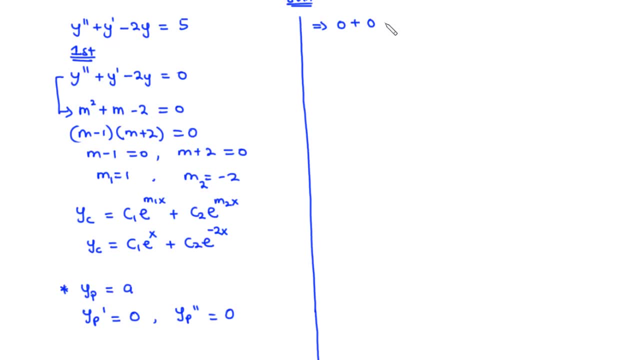 plus y prime, which is also zero, minus two times y, which is a, and that is equal to five. so next we have negative two: a equals five. we try to find the value of a, so we divide through by negative two, by negative two, and then you realize that we have a to be equal to negative five over. 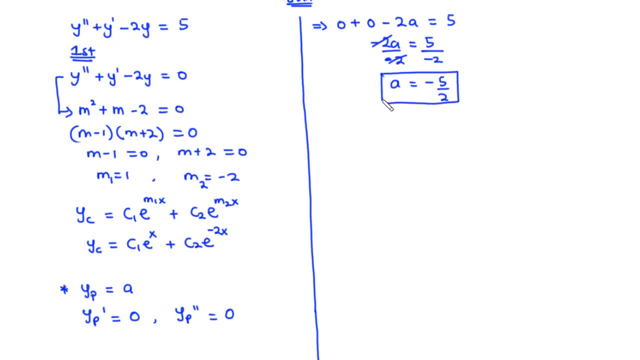 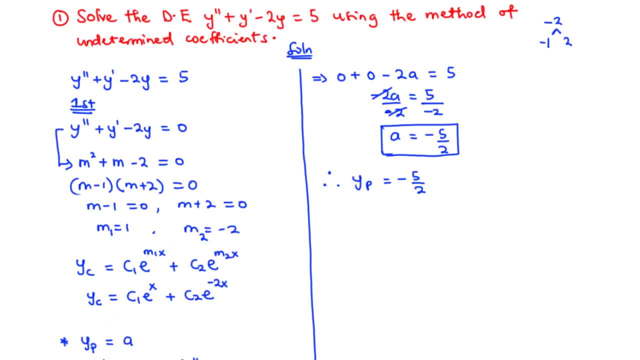 two. so this is the value of a. therefore we have the particular integral: yp equals a and a is negative five over two. now the general solution to the differential equation we know is given by y equals yc plus yp. and then we have yc to be c1, e to the power, x plus c2, e to the power, negative two x. 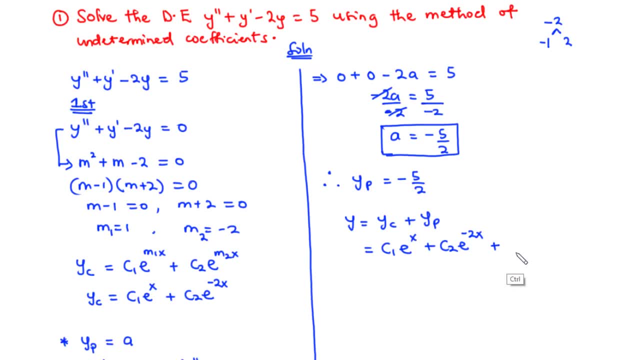 plus yp, which is negative five over two, so minus five over two. therefore we have the general solution to the differential equation to be: y equals c1 times e to the power, x plus c2 times e to the power. negative two x minus five over two. so now let's move on to the next example. 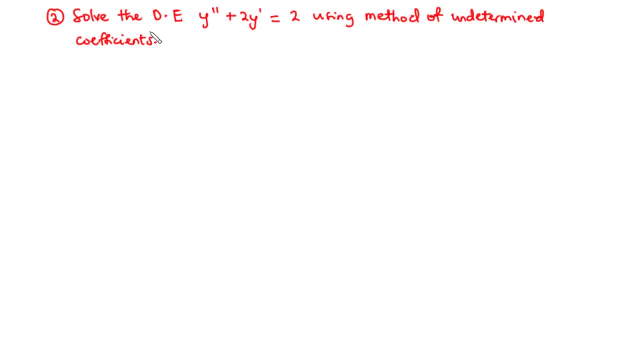 so, for example two, we are going to solve the differential equation y prime prime plus two- y prime equals two using the method of undetermined coefficients. so let's try to solve this example together. here we have y prime prime plus two, y prime equals two. now this differential equation is non-homogeneous, so we 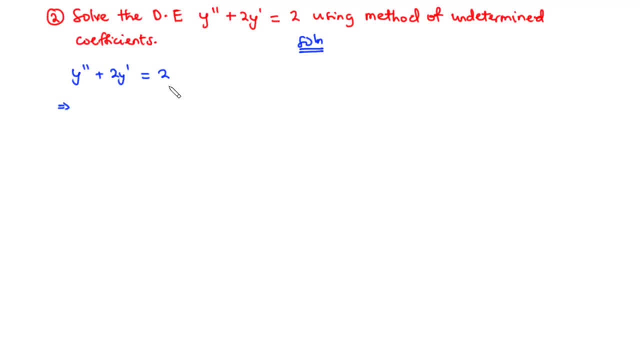 can make it homogeneous by equating or by making the right hand side equal to zero. okay, by making the right hand side equal to zero. so then we have y prime prime plus two. y prime equals zero. so this differential equation becomes homogeneous, and let's try to find the general solution of this. 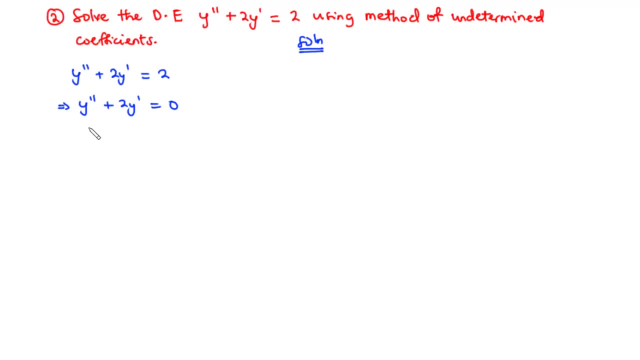 homogeneous differential equation. so we are going to represent y prime prime with m, square y prime with m, and thus we have this to be the auxiliary equation. so on the left hand side we can factor out m. so we factor out m. inside of the brackets we are going to have m plus two, so m. 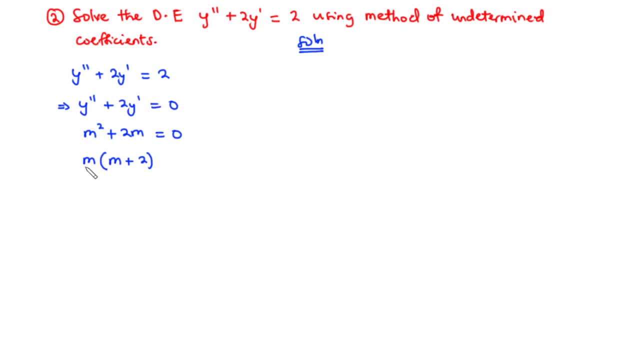 divided by m is m, and then two m divided by m is two. so we have this equal to zero. so here we have m equals zero. and then we have m plus two equals zero, so that we have m equals. we transpose this to the right hand side: we have negative two. so here we have m1 to be zero and then m2 to be. 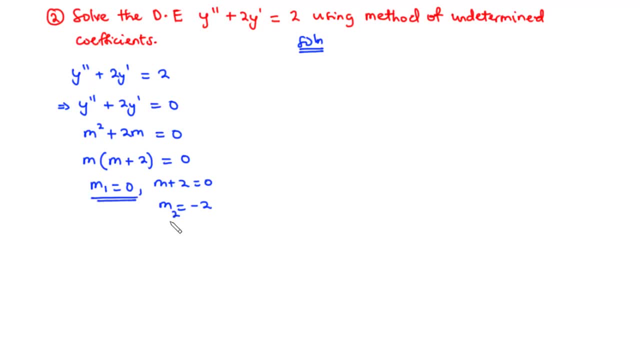 negative two. so these two roots are real and unequal. so we have the general solution of the homogeneous differential equation, giving us the complementary function equals c1 e to the power m1 x, plus c2 e to the power m2 x, so that becomes c1 e to the power. we have m1 to be zero. so zero times x is still zero. 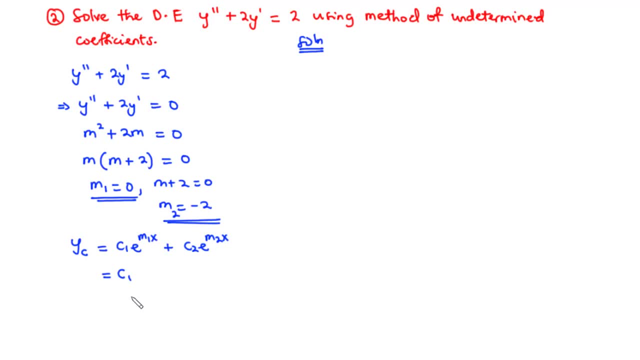 now e to the power, zero is equal to one. so therefore we have to have c1 times one, which is still c1. so plus c2 e to the power, this becomes negative two x. so this is the general solution of the homogeneous differential equation, the complementary. 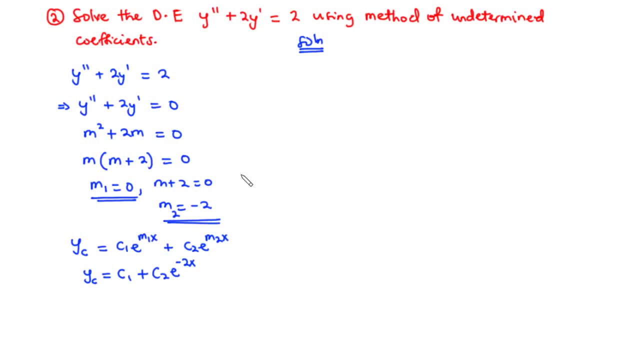 function. now let's try to find the particular integral. so for the particular integral, we are going to focus on the function g of x. that is the right hand side of this equation. so we have g of x to be two, and so under normal circumstance, because g of x is, a is a constant, then we deploy y: p equals a. now notice here, that's from the complementary. 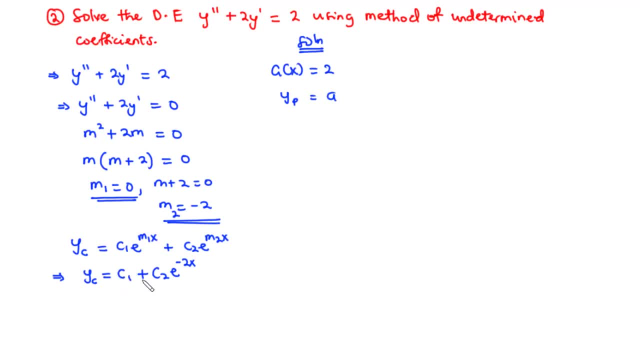 function we have a constant term, c1. now, whenever you have a constant term in the complementary function, then for the particular integral you are going to deploy yp equals ax instead of yp equals a. so you realize that in the previous example we deployed yp equals a, but in this example, because we have a constant term in the complementary function, we are going